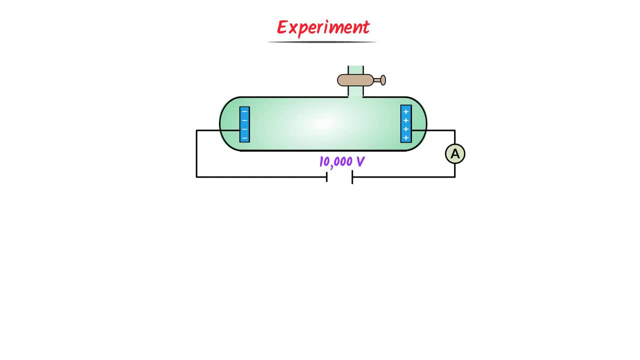 pressure. When we provide high voltage to it, we will see the continuous deflection of the ammeter. Now here you have to think like a scientist. Cathode and anode are not connected. I mean there is a gas between anode and cathode. We know that gas is an insulator and current doesn't pass. 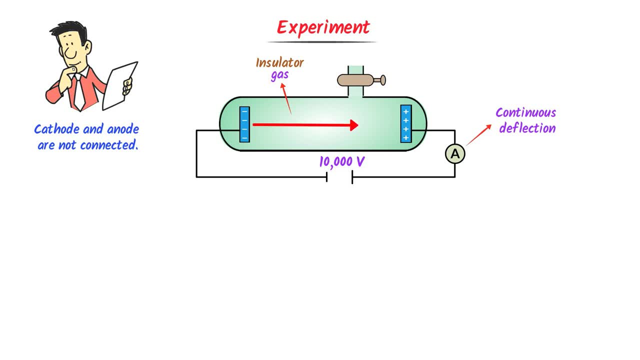 through the insulator, But we observe the continuous deflection of ammeter, which reveals that current is continuously flowing in the circuit. My question is: how current is passing through the glass tube? Well, we assume two possible solutions of this mystery. Firstly, we assume that the current 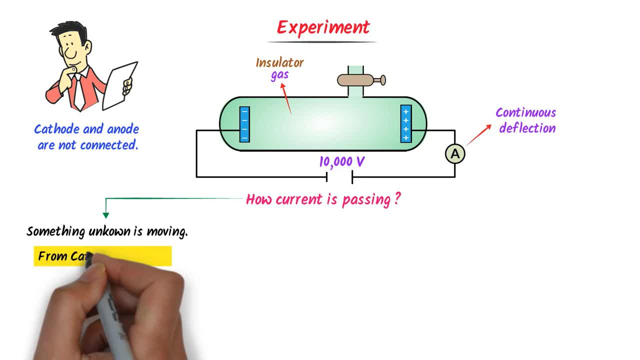 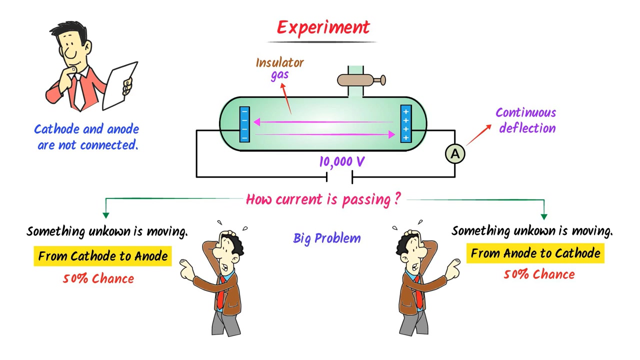 is moving from the anode towards the cathode. Secondly, we assume that something unknown is flowing from the cathode towards the anode. So there is 50% probability about this unknown flow. Now here we face big problem. I mean, we are not sure that in which direction this unknown thing is. 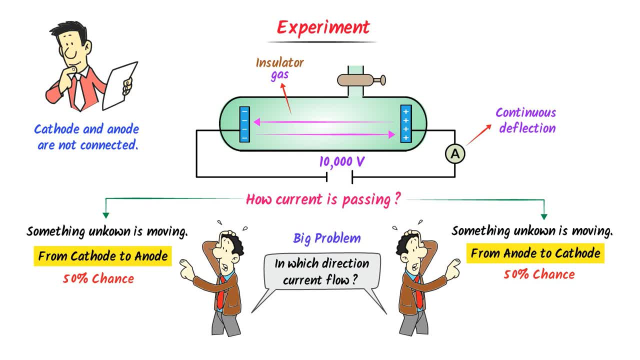 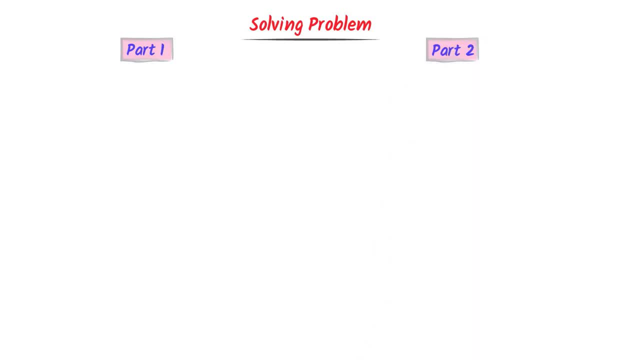 flowing. I mean, can we detect the flow of unknown thing or current? Well, we will solve this problem in two parts. In the first part, we take the discharge tube. We create a small hole in the cathode. Secondly, we coat the back side of the cathode by fluorescent or zinc sulfide. 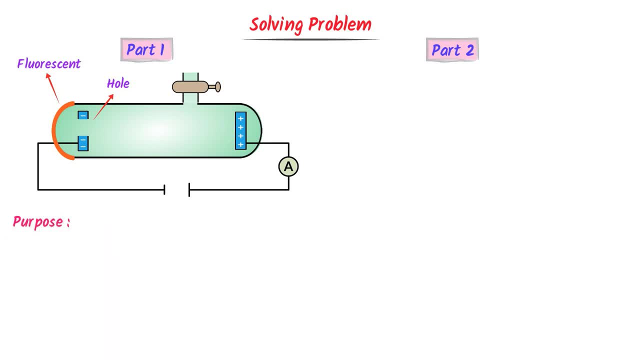 Now, what is the purpose of this hole and fluorescent screen? Well, its purpose is simple. I mean, if something is flowing from anode towards the cathode, it may pass through this hole and may hit the fluorescent screen. As a result, we will see a glow on the fluorescent. 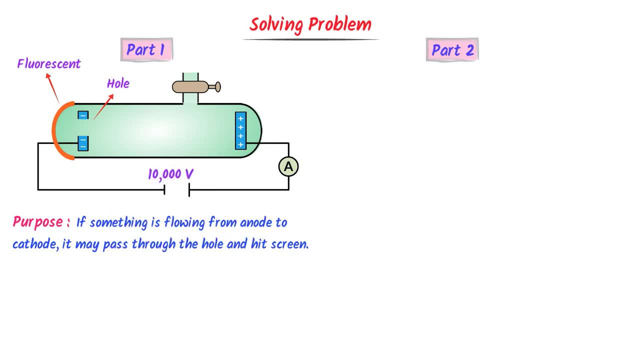 screen. Now we will provide the high voltage. The ammeter shows continuous deflection. It means that current is passing through the circuit, But the result is nothing. I mean we do not detect the diffusers like any other, force出去 any thing or any glow on the fluorescent screen. 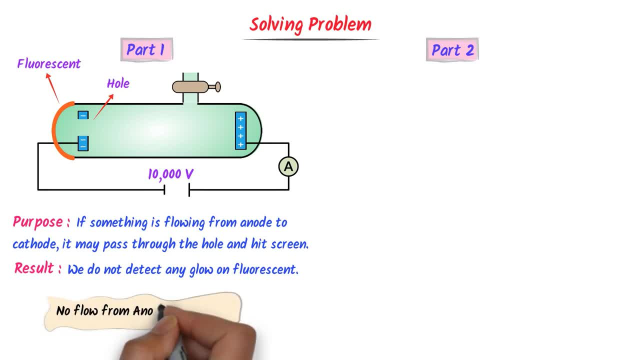 Hence we say that the unknown thing is not flowing from anode towards cathode on a constant flow. This assumption, or part one, is badly failed. We discovered nothing. Now, in the second part, we do the opposite experiment. We take this discharge tube, We create small hole in the anode. 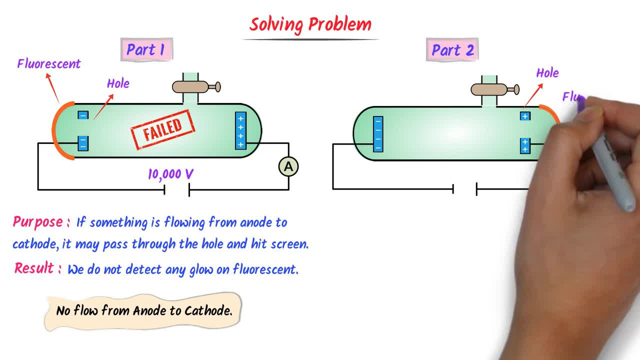 Secondly, we coat the big side of the anode byублиking on the cathode. Now, what is the function by fluorescent or zinc sulfide? Its purpose is simple. If something is flowing from the cathode towards the anode, it may pass through this hole and may hit the fluorescent screen. 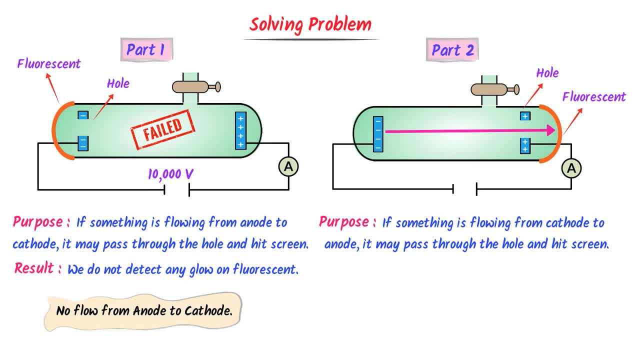 As a result, we will see a glow on the fluorescent screen. Now we will provide high voltage. The emitter shows continuous deflection. It means that current is passing through the circuit. But the result is stunning. I mean we see glow on the fluorescent screen. Congratulations. 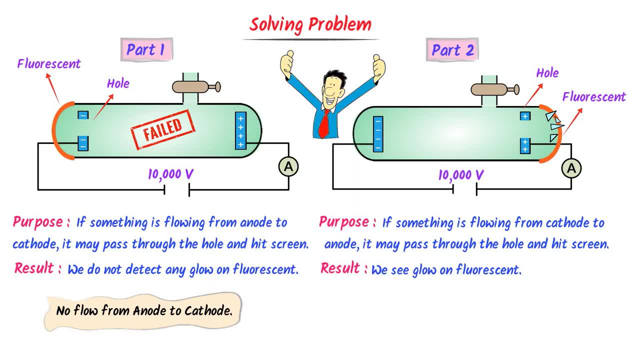 everyone. We have solved the problem. This glow on the fluorescent screen means that something unknown is moving in straight line from the cathode towards the anode. Let me repeat it: This glow on the fluorescent screen means that something is moving in straight line from the cathode towards the anode. 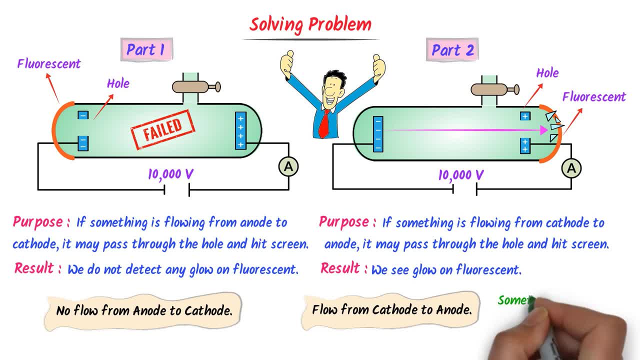 We call this something unknown as cathode rays. Remember that we call this cathode ray because these rays originate, are produced from the cathode. Thus we learn that cathode rays are produced in this discharge tube, which causes the emitter to deflect and current is continuously flowing in the circuit. Thus we successfully solved this problem. Now we 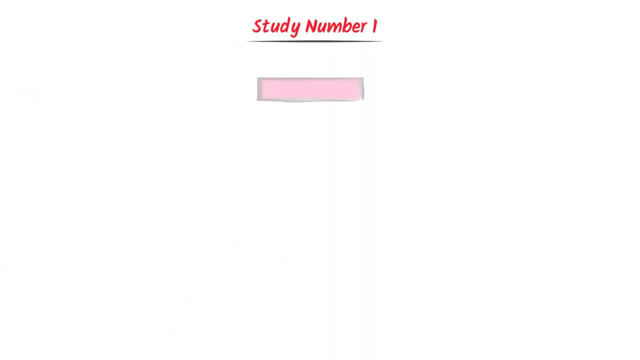 will further study the emitter Now. we will further study the emitter Now. we will further study the emitter Now. we will consider the behavior of the cathode rays. Consider this electric field. I am interested to pass the cathode rays through this electric field. After passing the cathode rays through, 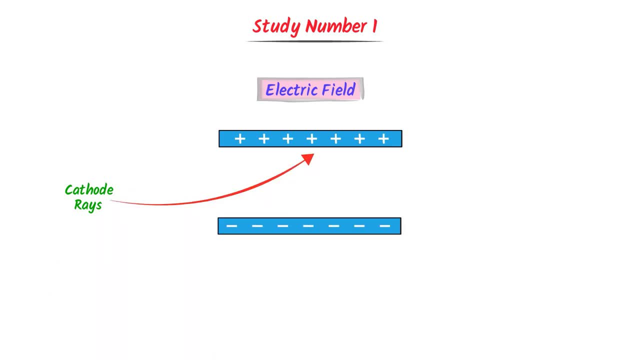 the electric field, we observe that the cathode rays bend towards the positive plate. We know that the opposite charge attracts The cathode ray bends towards the positive plate and electric field because they are negatively charged. Let me repeat it Now: we know that the cathode 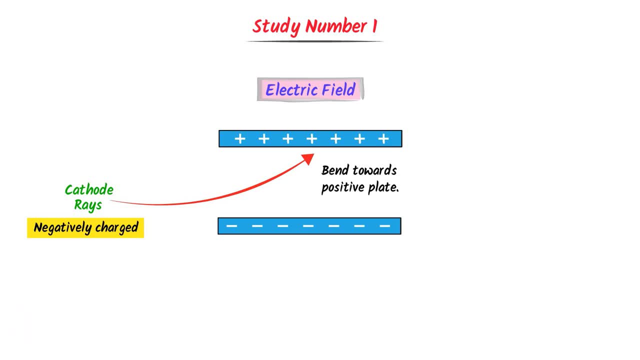 Ketaud rays bend towards positive plate and electric field because they are negatively charged. So we learn that Ketaud rays are negatively charged. Also, remember that Ketaud rays deflect an electric field and a magnetic field. In absence of electric and magnetic field, they will move in a straight line. 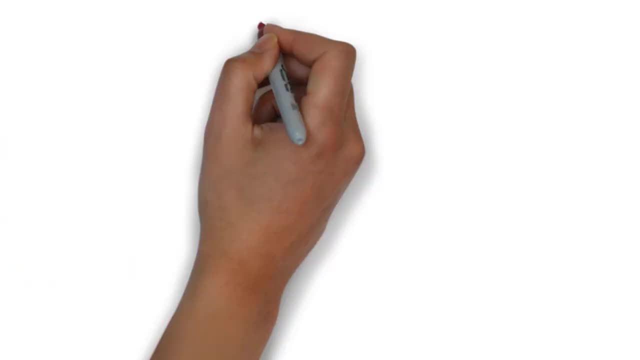 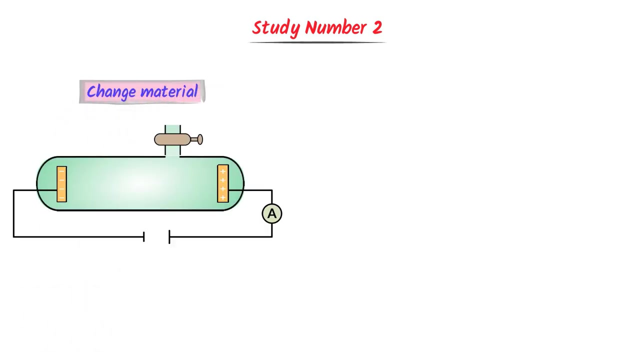 Hence noted down these important points. Now we will further study the behavior of Ketaud rays in the second study. In this study we change the material of both the Ketaud and Inode When we provide high voltage. we observe that the same Ketaud rays are produced in this. 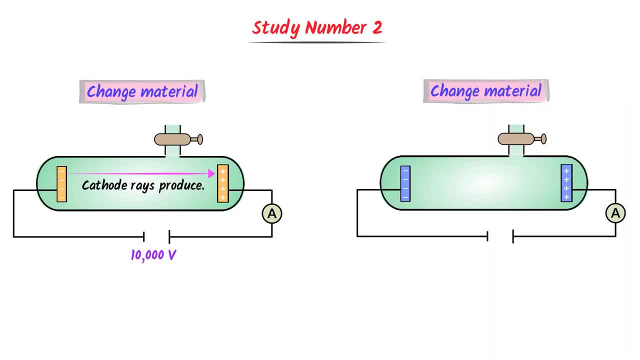 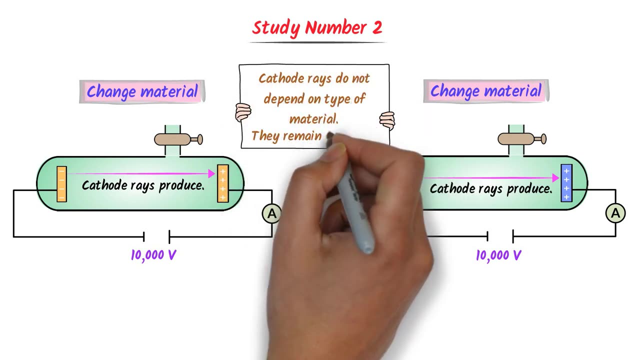 glass tube. Secondly, we again change the material of both Ketaud and Inode. Again we observe that the same Ketaud rays are produced. So we say that the same Ketaud rays are produced in this glass tube. We also say that Ketaud rays do not depend on the type of material. they are same for. 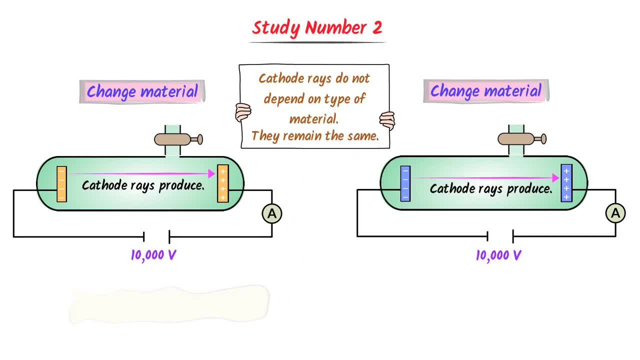 all materials. Hence we conclude that Ketaud rays are nothing but a stream of electron or sea of electrons. Secondly, we conclude that Ketaud rays are the basic constituent particles of all materials, because all the different materials produce Ketaud rays. 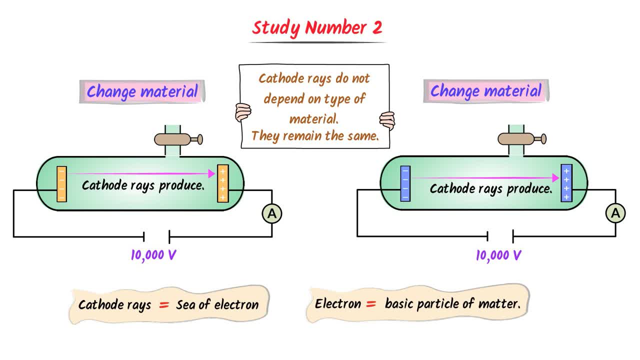 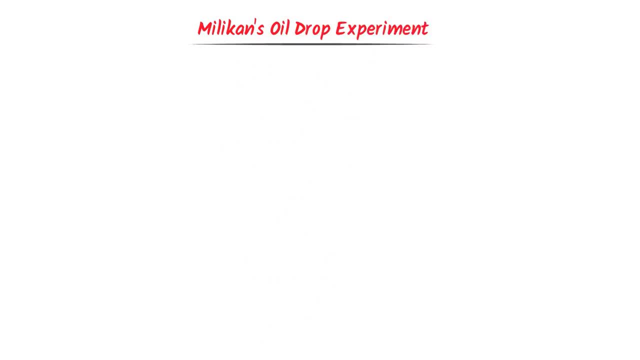 Thus remember that We discover Ketaud rays, which is made up of electrons. Now, in the third study of Millikan oil-drop experiment, we can easily calculate the charge of electron, which is equal to 1.6 x 10 to the power negative 19 coulomb. 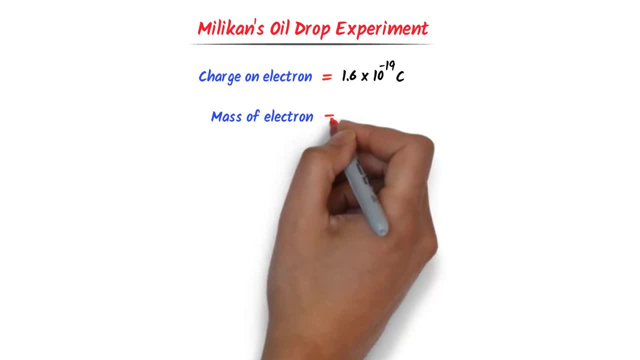 Also, we calculate the mass of electron, which is equal to 9.1 x 10 to the power negative, 31 kg. Remember that. So when we calculate the charge of electron, we already consider the charge of electron to be equal to 1.6 x 10 to the power negative 19 coulomb. 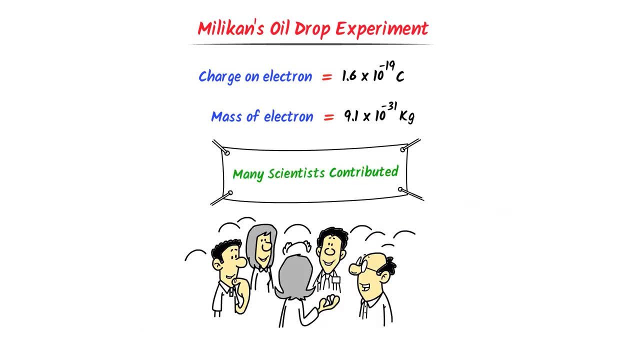 electron is a long process and many scientists contributed in this discovery, but the whole credit goes to JJ Thomson. That's why we say that JJ Thomson discovered electron. Thus, from all these studies we conclude that the cathode ray starts from cathode and move towards.